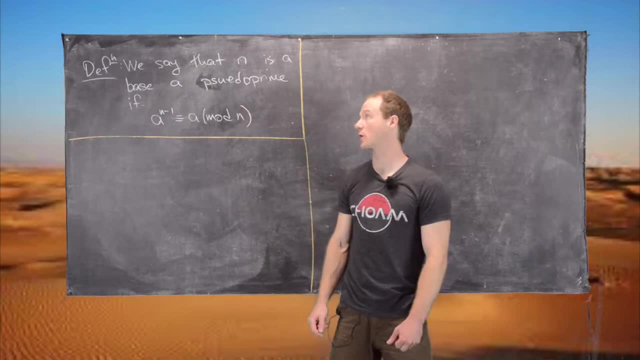 Okay, in this video we're going to look at the notion of a pseudoprime number, And so in fact we're going to look at a special type of pseudoprime number called the Fermat pseudoprime. So let's recall, Fermat's little theorem says that if you have a prime p and a number that's relatively prime to p, 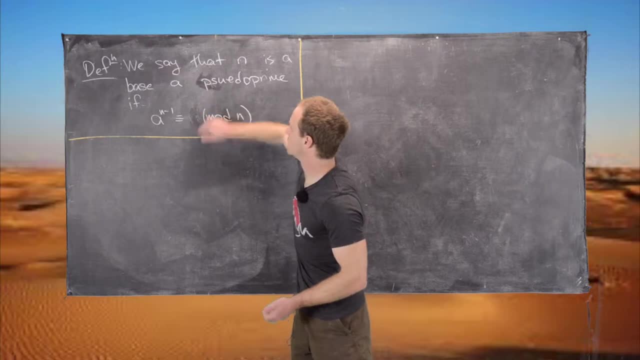 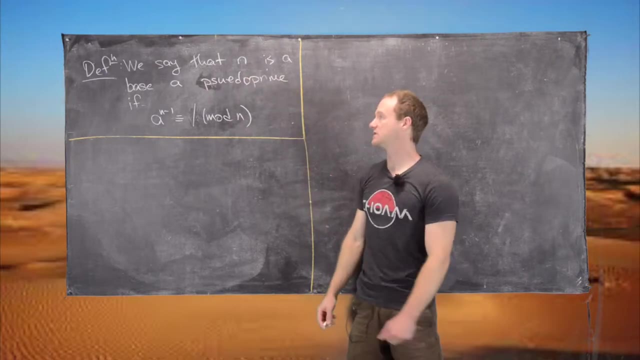 a to the p minus 1 is congruent to 1 mod p, And so that gives us this motivation. We say that n is a base, a pseudoprime, if a to the n minus 1 is congruent to 1 mod n. 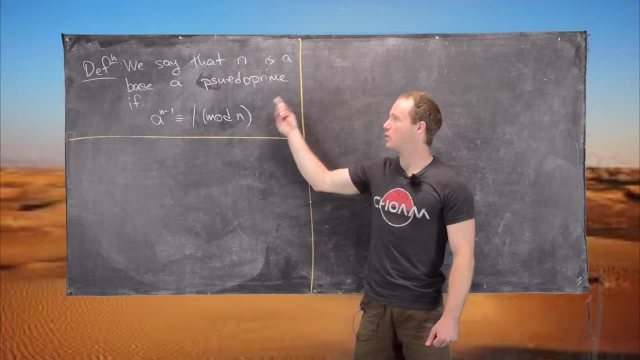 So let's just like see, maybe, why it would be called a pseudoprime, because it acts like something having to do with Fermat's little theorem, But in fact it may not be a prime number. So let's look at an example. 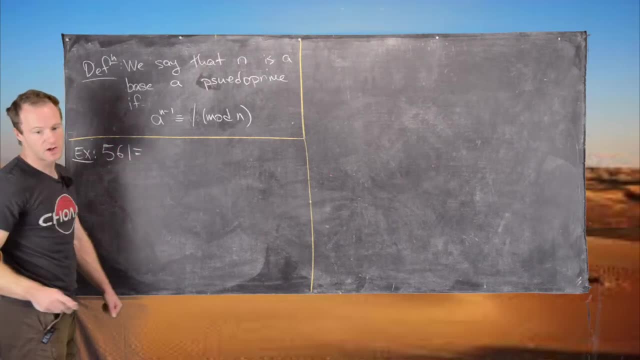 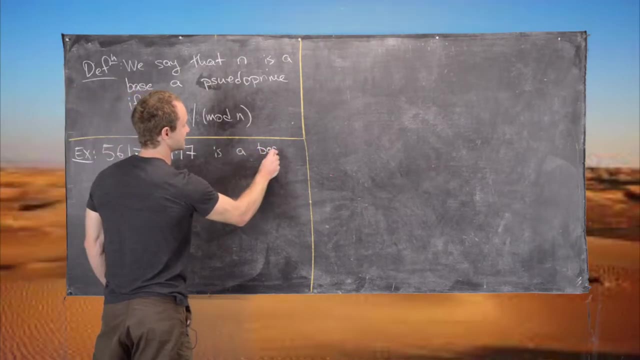 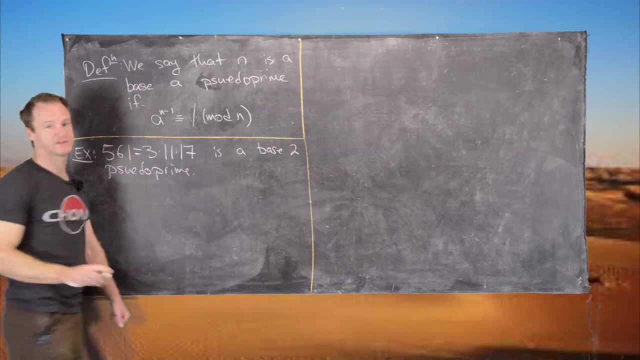 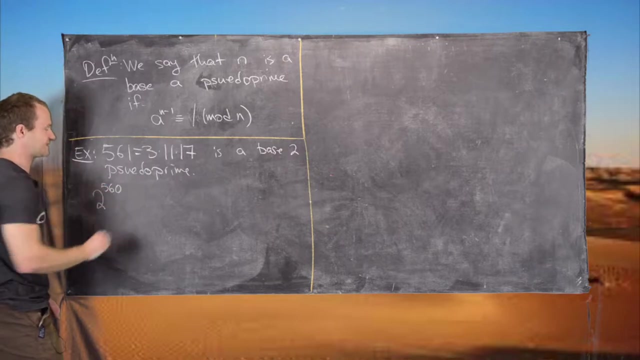 So an example: So 561, which is equal to 3 times 11 times 17, is a base 2 pseudoprime. So let's check that. So we need to look at 2 to the power 560.. 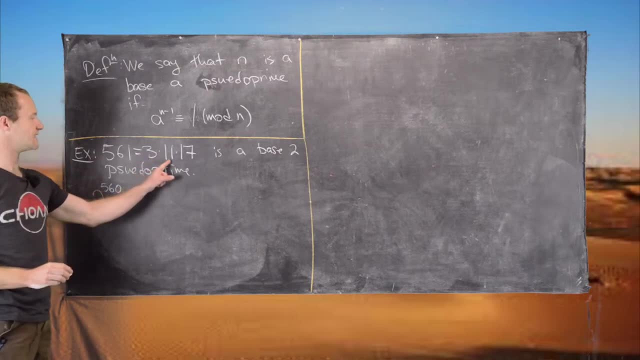 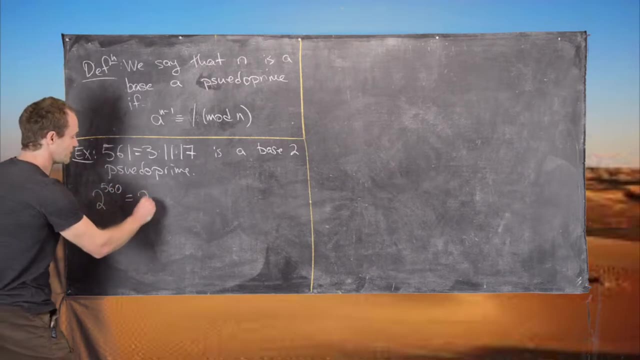 And what we'll do is look at this mod, all of these individual components of the number 561.. So notice that this is equal to 2 to the power, 2 to the power 280.. But 2 to the 2 is congruent to 1 mod 3 by Fermat's little theorem. 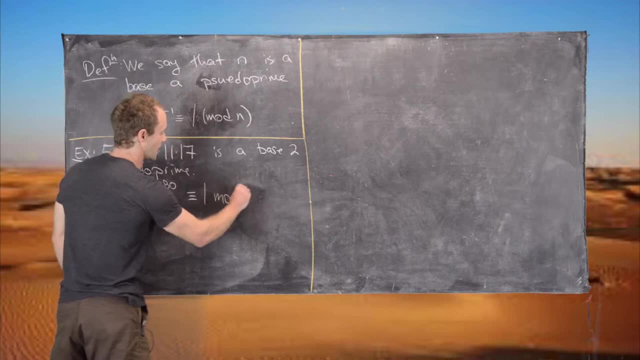 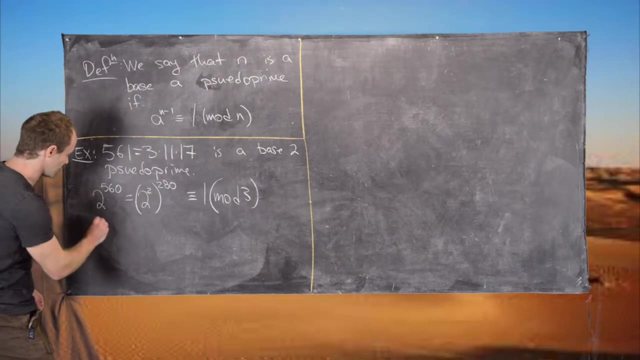 So that means this whole thing is congruent to 1 mod 3.. Again by Fermat's little theorem, with 3 being the prime. Next we want to look at 2 to the 560, which is equal to 2 to the 10 to the 56.. 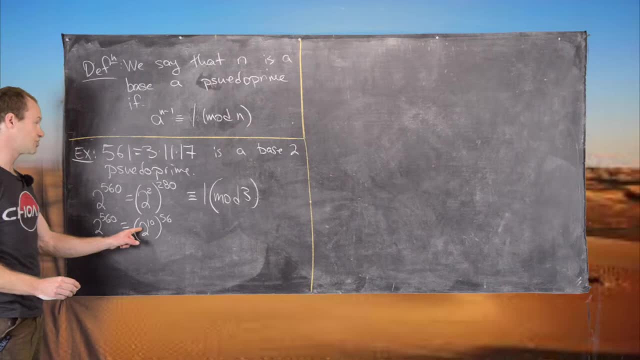 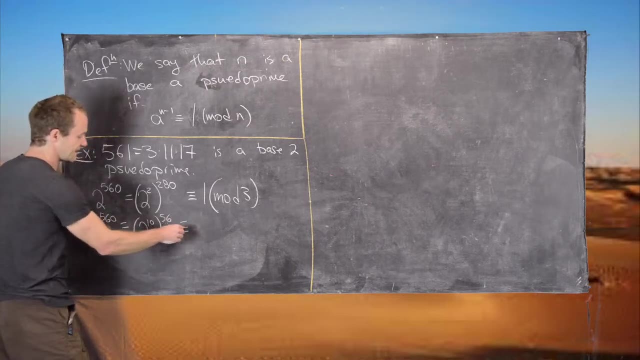 And again, because 11 is a prime and 2 is relatively prime to 11, 2 to the 10 is congruent to 1 mod 11.. Which means 2 to the 10 to the 56 is 1 to the 56, which is 1 mod 11, again by Fermat's little theorem. 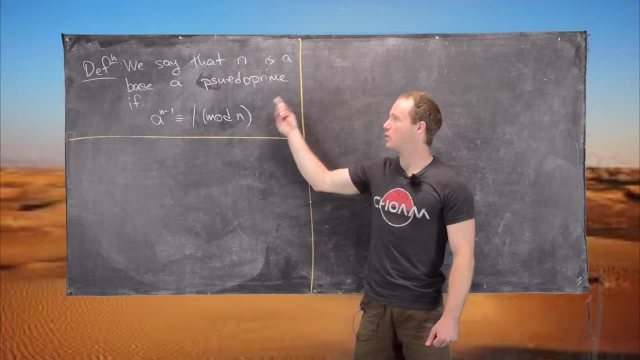 So let's just like see, maybe, why it would be called a pseudoprime, because it acts like something having to do with Fermat's little theorem, But in fact it may not be a prime number. So let's look at an example. 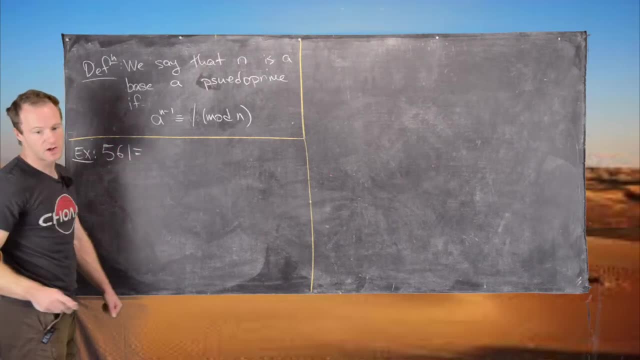 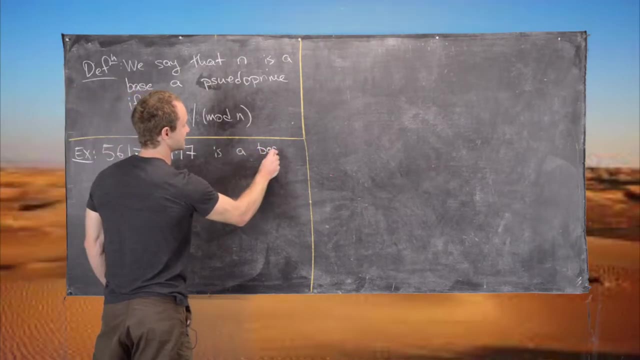 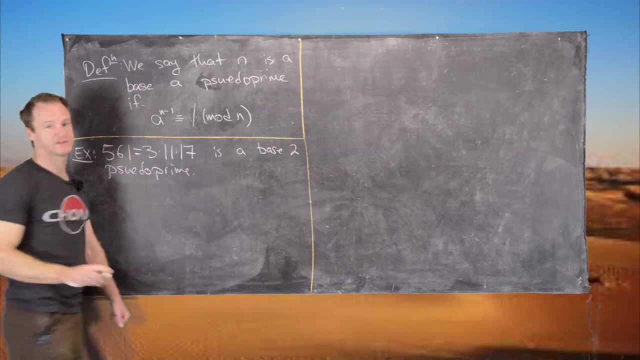 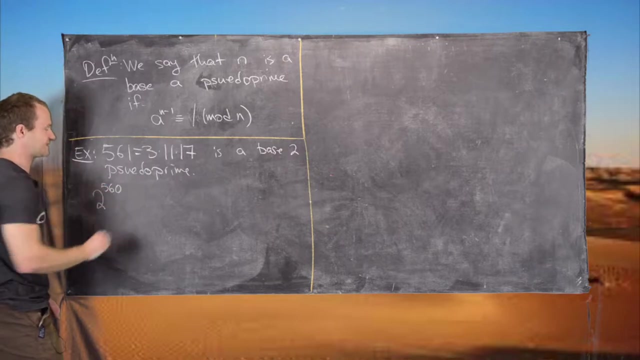 So an example: So 561, which is equal to 3 times 11 times 17, is a base 2 pseudoprime. So let's check that. So we need to look at 2 to the power 560.. 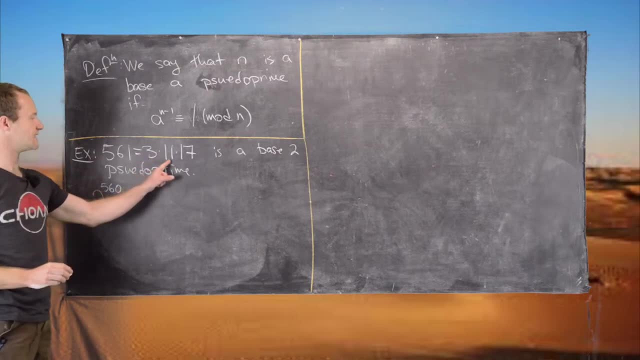 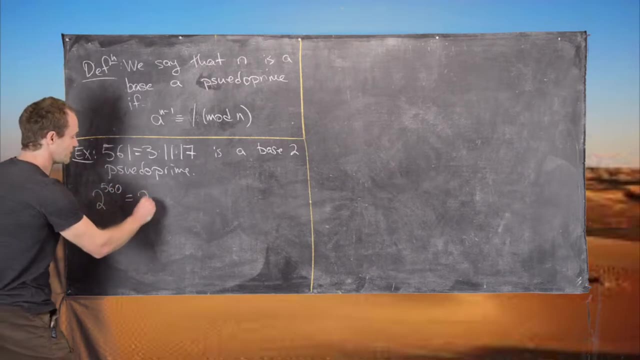 And what we'll do is look at this mod, all of these individual components of the number 561.. So notice that this is equal to 2 to the power, 2 to the power 280.. But 2 to the 2 is congruent to 1 mod 3 by Fermat's little theorem. 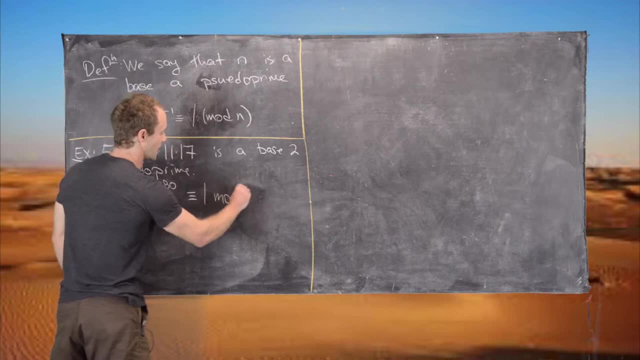 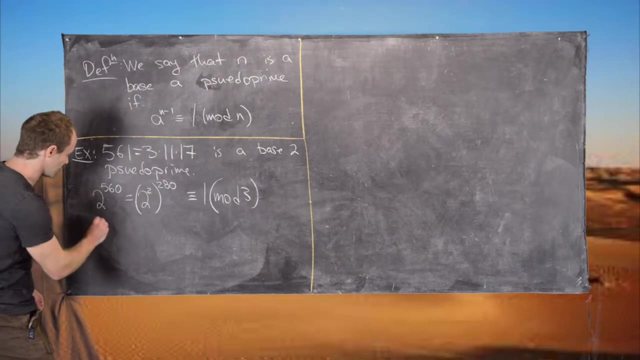 So that means this whole thing is congruent to 1 mod 3.. Again by Fermat's little theorem, with 3 being the prime. Next we want to look at 2 to the 560, which is equal to 2 to the 10 to the 56.. 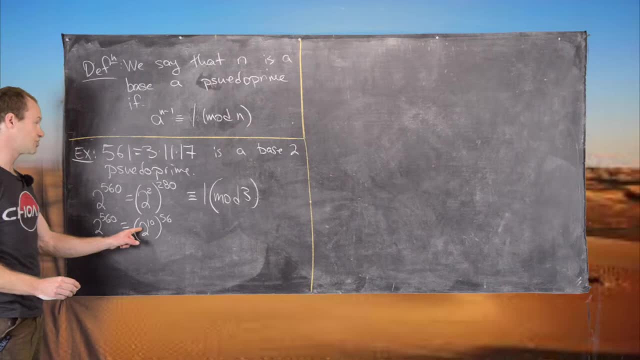 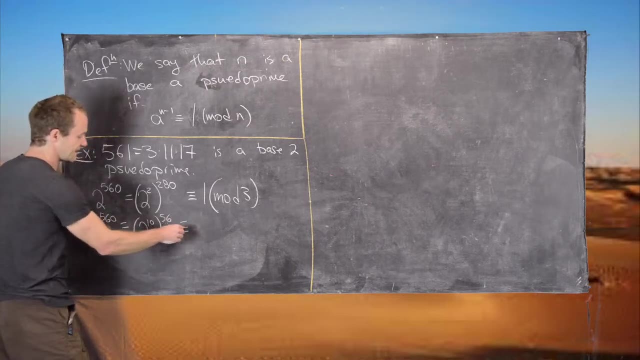 And again, because 11 is a prime and 2 is relatively prime to 11, 2 to the 10 is congruent to 1 mod 11.. Which means 2 to the 10 to the 56 is 1 to the 56, which is 1 mod 11, again by Fermat's little theorem. 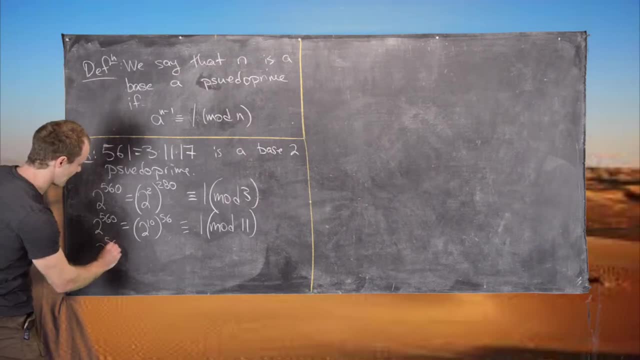 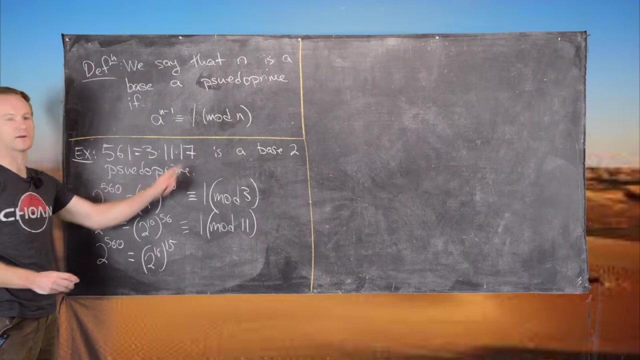 Great, And finally we have 2 to the 560 is going to be 2 to the 16, to the power 15.. Good, And again, 2 to the 16 is congruent to 1 mod 17 by Fermat's little theorem. 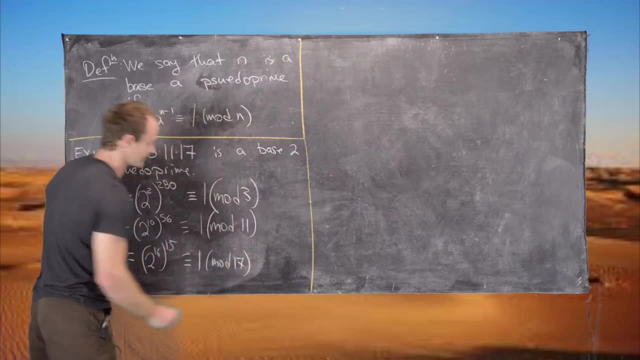 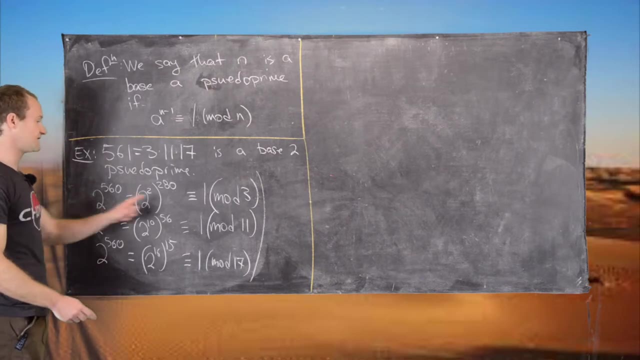 So this whole thing is 1 mod 17.. Good, And now putting all of these things together, So if 2 to the 560 is congruent to 1 mod 17, by Fermat's little theorem, 560 is 1 mod 3,, 2 to the 560 is 1 mod 11, and 2 to the 560 is 1 mod 17, then it follows that 2. 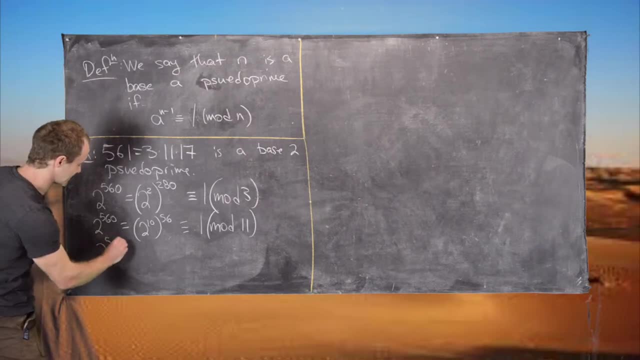 Great, and finally we have. 2 to the 560 is going to be 2 to the 16, to the power 15.. Good and again, 2 to the 16 is congruent to 1 mod 17 by Fermat's little theorem. 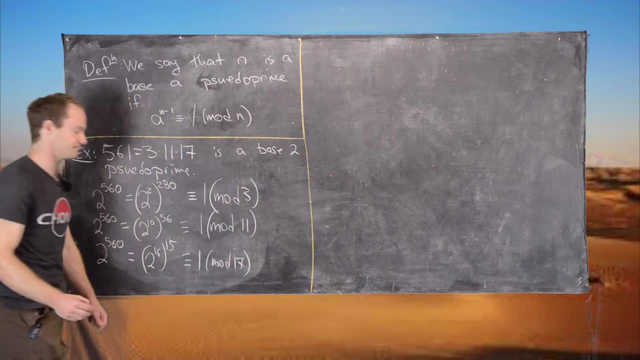 So this whole thing is 1 mod 17.. Good, and now putting all of these things together, So if 2 to the 560 is congruent to 1 mod 12, then this whole thing is congruent to 1 mod 17 by Fermat's little theorem. 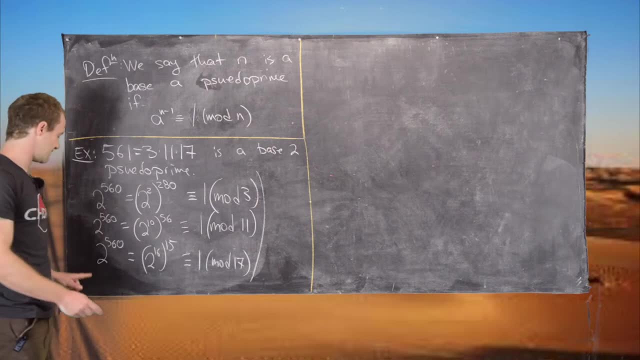 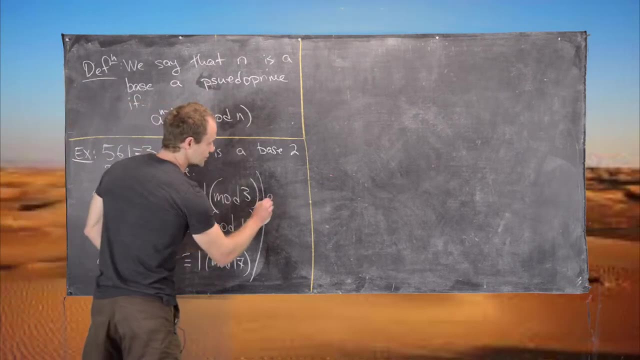 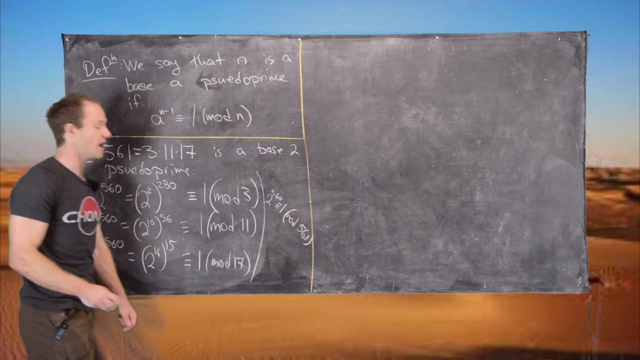 560 is 1 mod 3,, 2 to the 560 is 1 mod 11, and 2 to the 560 is 1 mod 17,. then it follows that 2 to the 560 is congruent to 1 mod 561.. In other words, 561 is a base 2 pseudoprime. Okay, let's look at. 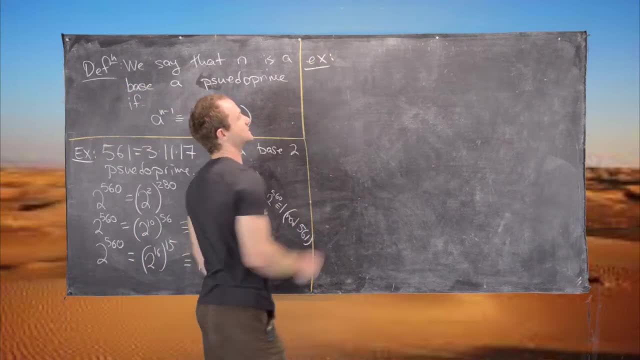 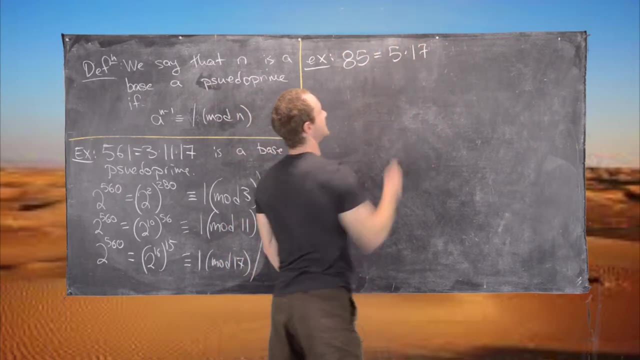 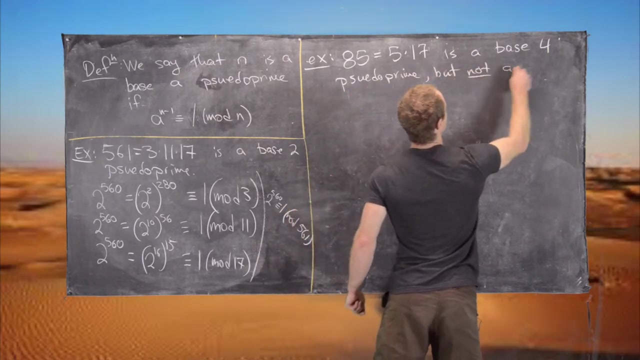 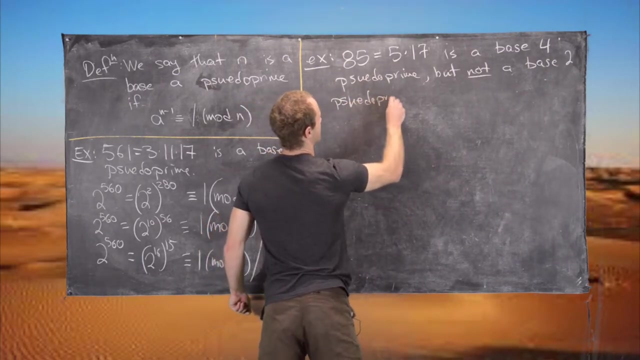 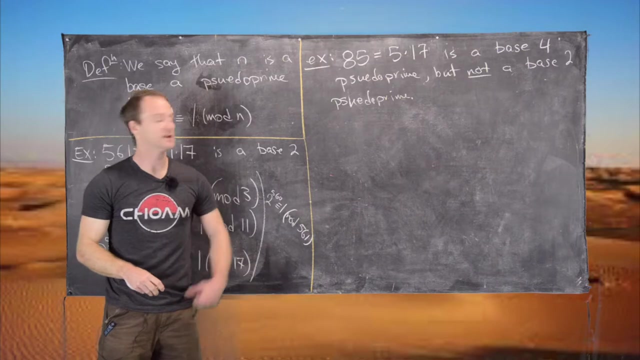 another example. So the next example is 85,, which equals 5 times 17, is a base 4 pseudoprime but not a base 2.. So I think it's interesting that this one is a base 4 pseudoprime but not a base 2 pseudoprime. 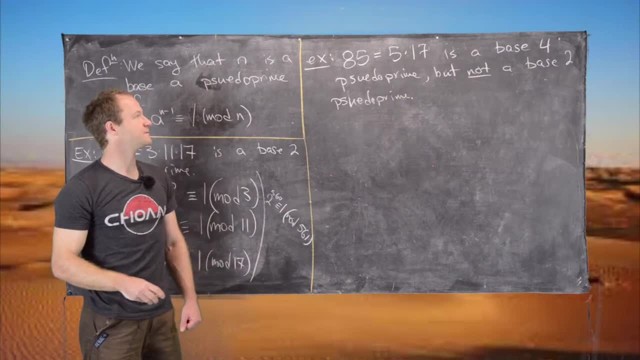 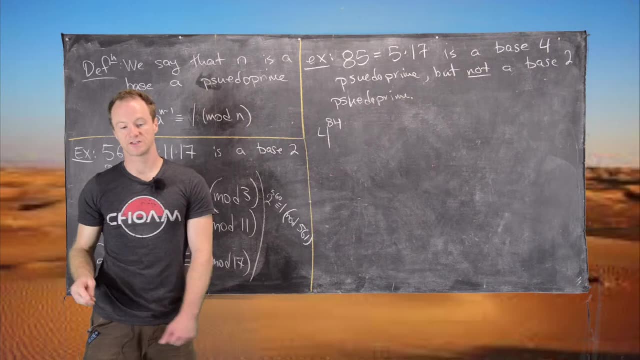 So that's why I'm including it as an example. Okay, so let's look at this: So we'll take 4 to the 84, and so we can write that as 4 to the 4 to the power 21,, and then we know 4 to the 4 is. 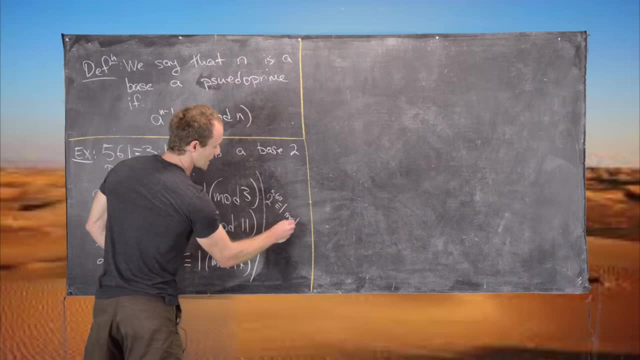 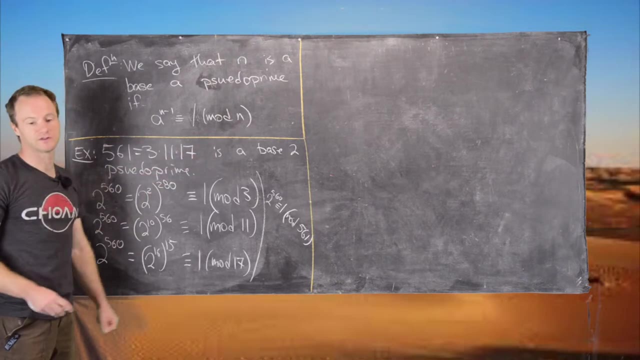 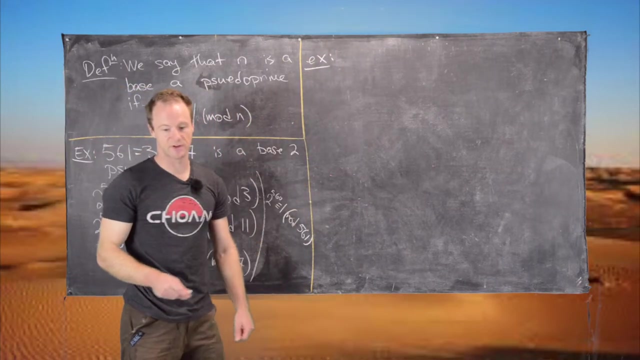 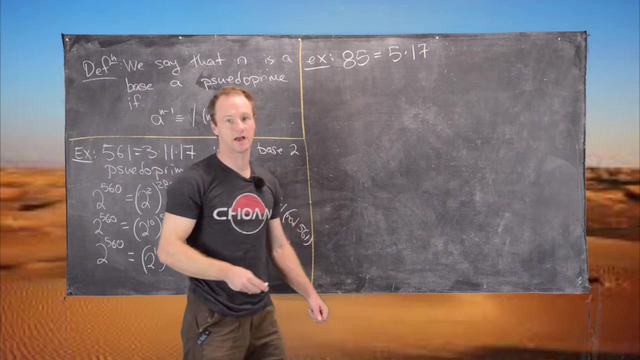 to the 560 is congruent to 1 mod 561.. In other words, 561 is a base 2 pseudoprime. Okay, let's look at another example. So the next example is 85,, which equals 5 times 17,, is a base 4 pseudoprime. 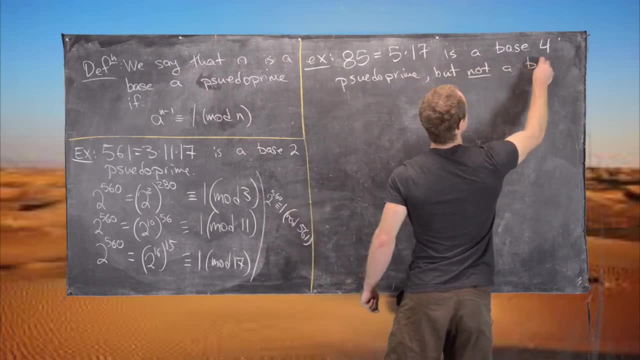 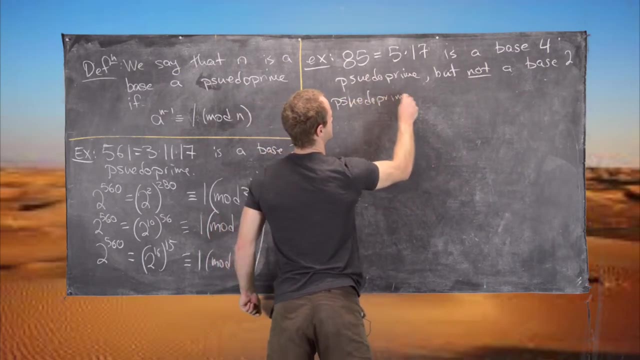 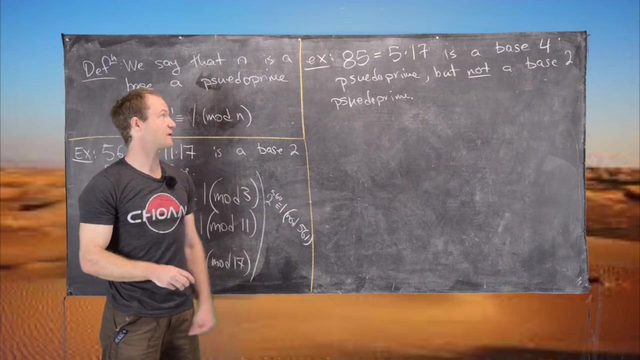 but not a base 2.. So I think it's interesting that this one is a base 4 pseudoprime but not a base 2 pseudoprime, so that's why I'm including it as an example. Okay, so let's look at this. So we'll take 4 to. 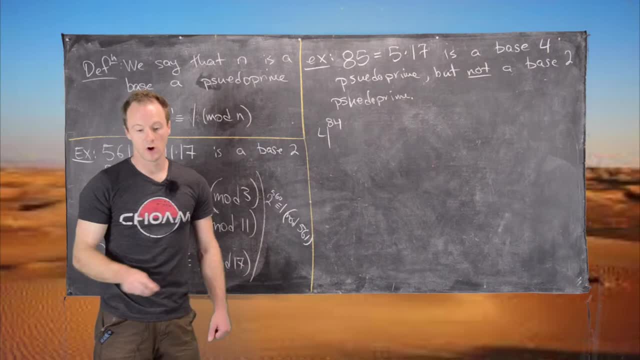 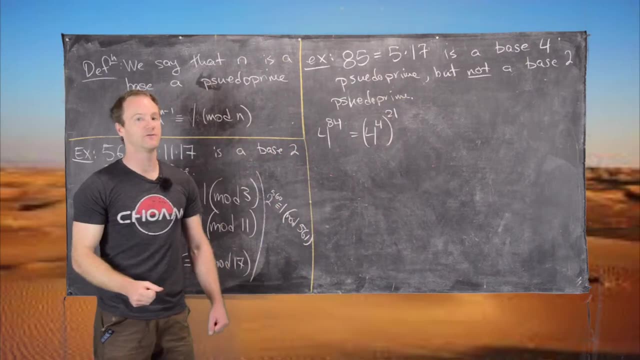 the 84, and so we can write that as 4 to the 4 to the power 21,, and then we know 4 to the 4 is congruent to 1 mod 5.. Again, we can write that as 4 to the 4 to the power 21,, and then we know 4 to the 4 is congruent to 1 mod 5.. 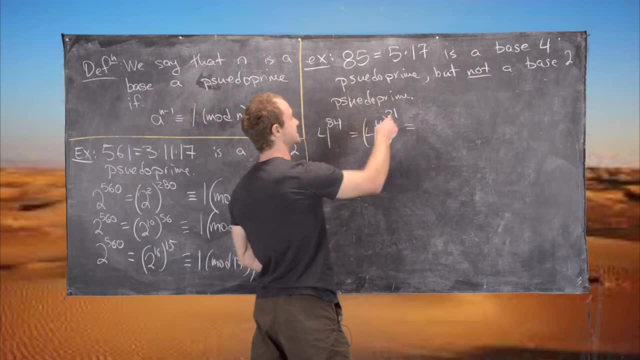 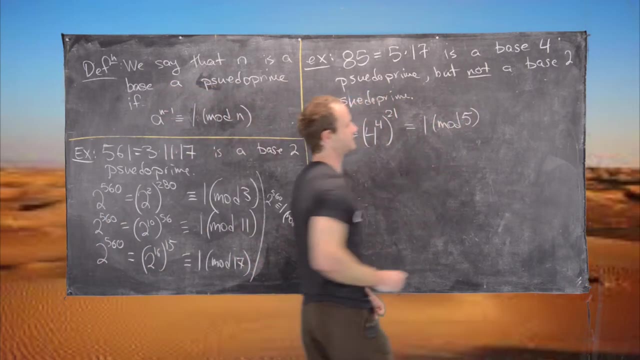 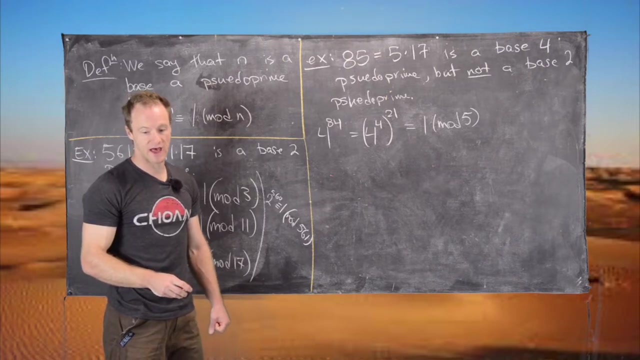 Again, we know: 4 to the 4 is congruent to 1 mod 5. Again by Fermat's Little Theorem. so this whole thing is 1 to the 21,, which is 1 mod 5.. Good, and now we'll work mod 17.. So let's do that. So we'll do 4 to the 84, and so if we work mod 17,, 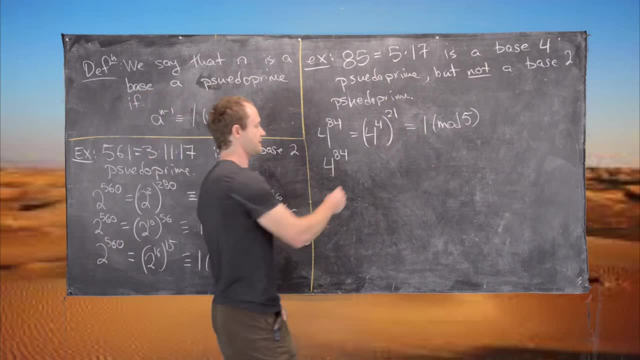 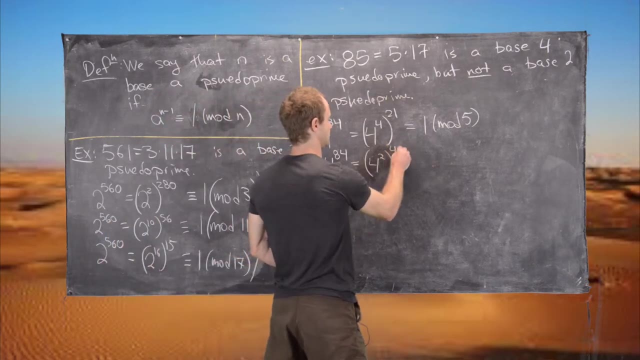 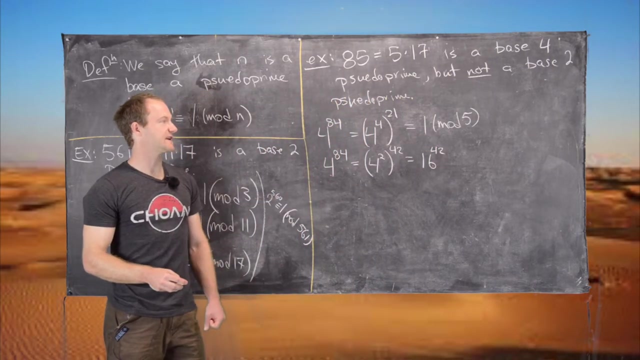 I'm actually going to use a little bit different of a trick here. So this is equal to 4, squared to the 42,, which is equal to 16 to the 42,, but now 16 is congruent to negative 1 mod 17,. 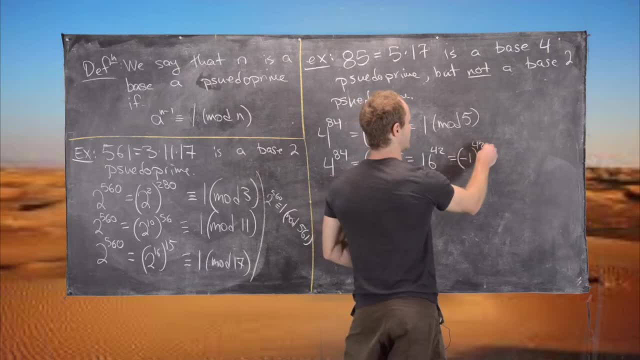 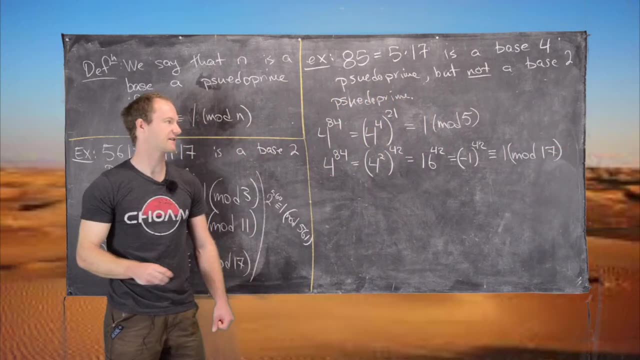 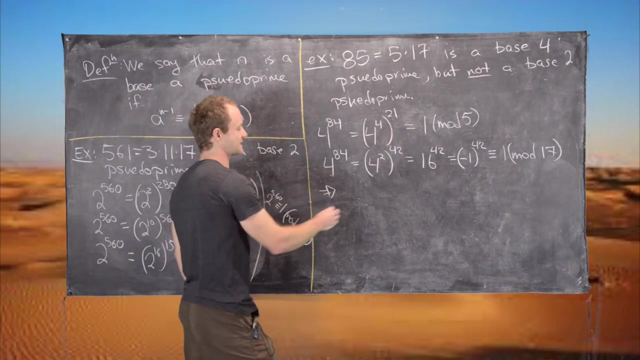 so that means this is equal to negative 1 to the 42,, which is congruent to 1 mod 17.. So there I use the fact that 16 is congruent to negative 1 mod 17.. Good, so all this together, these two facts, tell us that 4 to the 84 is congruent to 1 mod. congruent to 1 mod 5, again by 4.. So we can write that as 4 to the 4 to the power 21,. and then we know: 4 to the 4 is congruent to 1 mod 5,, again by 4.. 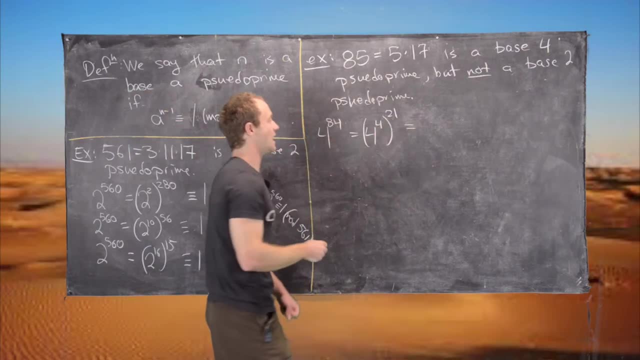 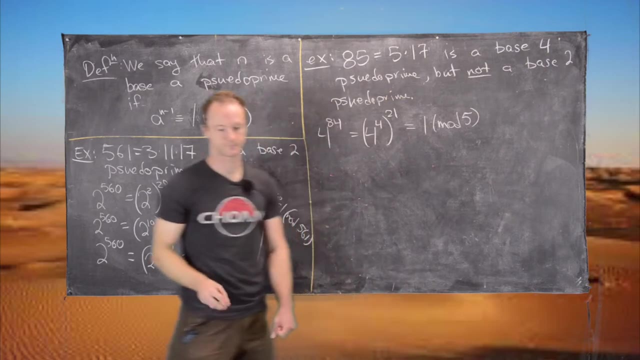 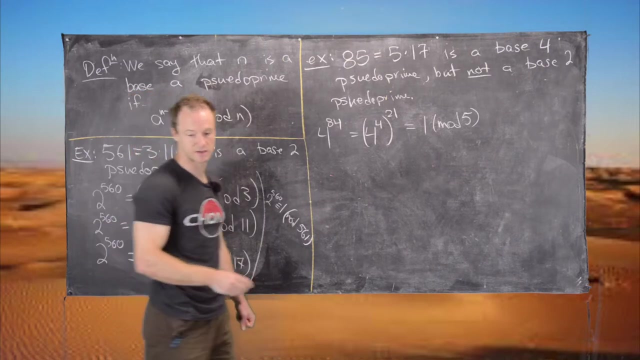 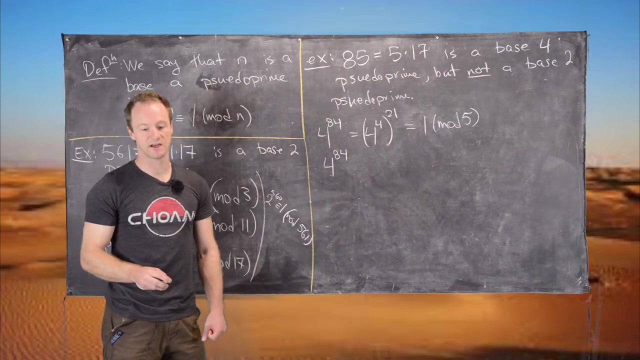 mod's little theorem. so this whole thing is 1 to the 21, which is 1 mod 5. good, and now we'll work mod 17, so let's do that. so we'll do 4 to the 84, and so if we work mod 17, I'm actually going to. 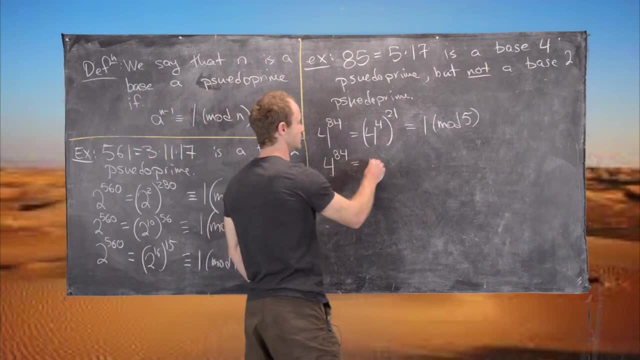 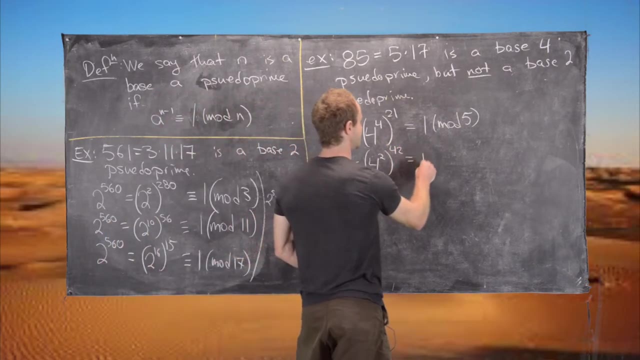 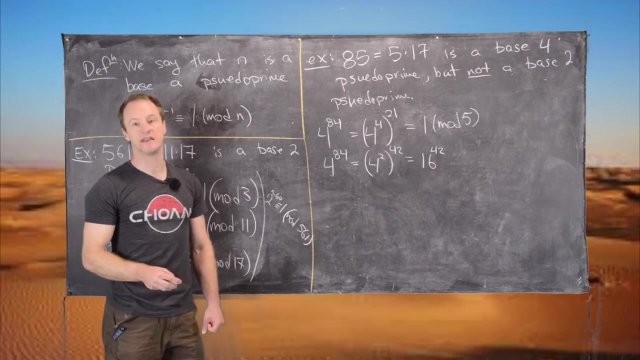 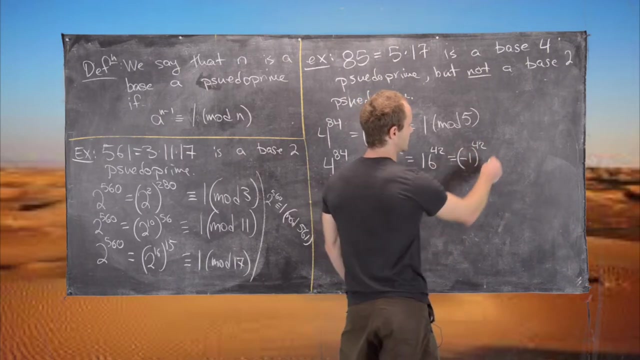 use a little bit different of a trick here. so this is equal to 4 squared to the 42, which is equal to 16 to the 42. but now 16 is congruent to negative 1 mod 17. so that means this is equal to negative 1 to the 42, which is congruent to 1 mod 17. so there. 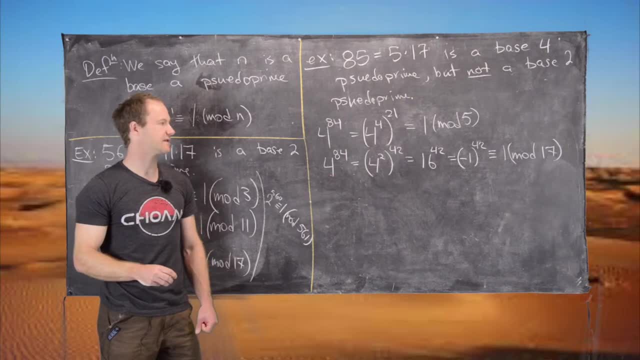 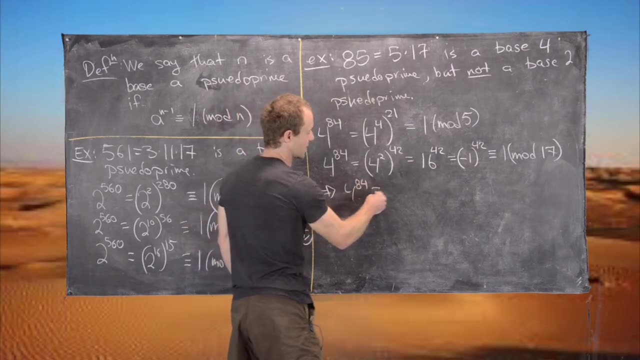 I go. I use the fact that 16 is congruent to negative 1 mod 17. good so, all this together, these two facts tell us that 4 to the 84 is congruent to 1 mod the product of 5 and 17, which is 18, sorry, 85. 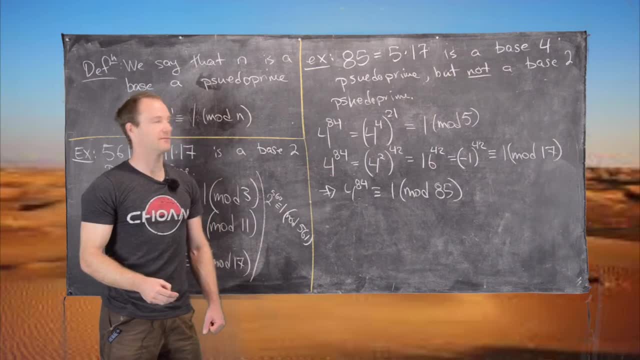 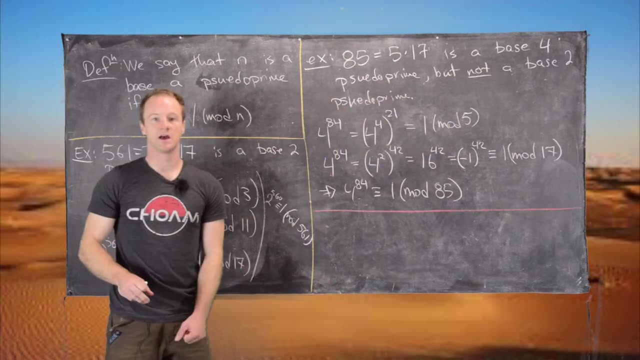 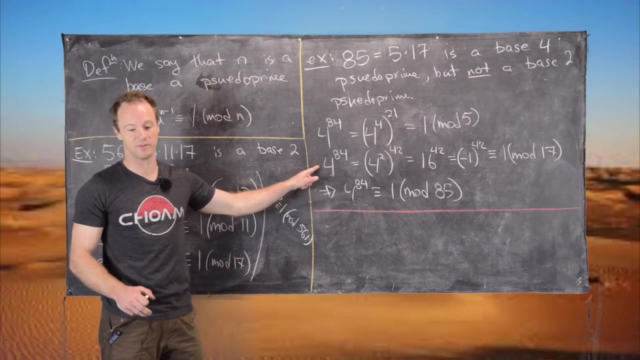 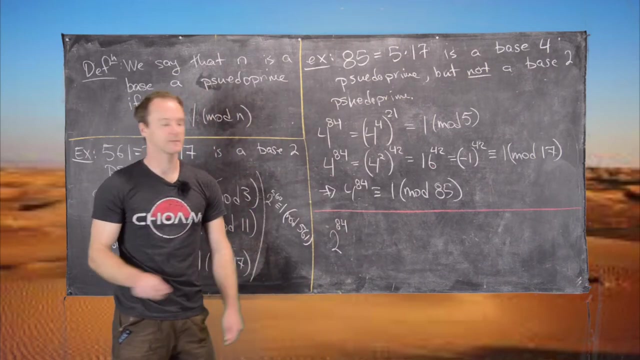 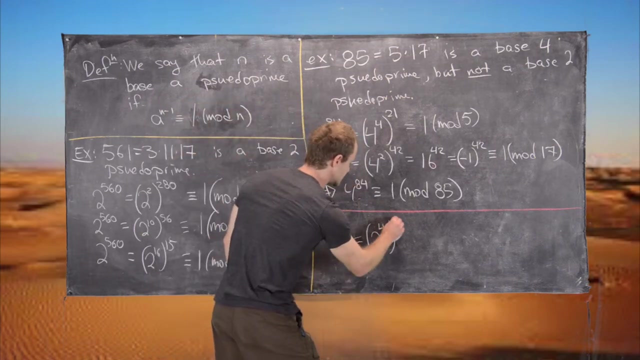 which means that 85 is a base 4 pseudoprime. okay, good. so now let's show why it's not a base 2 pseudoprime. so nothing will go wrong here. what will go wrong? and this is in this type of equation. so now let's look at 2 to the 84 and notice that 2 to the 84 is equal to 2 to the 4 to the 21. but 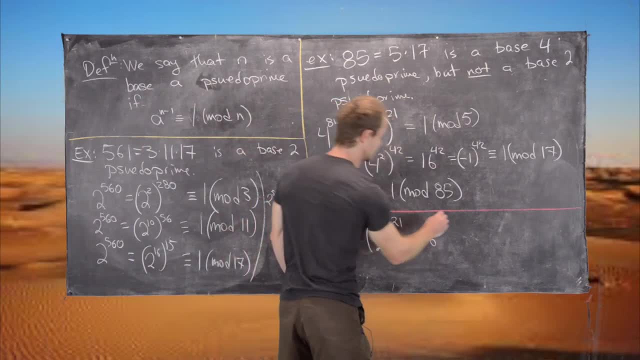 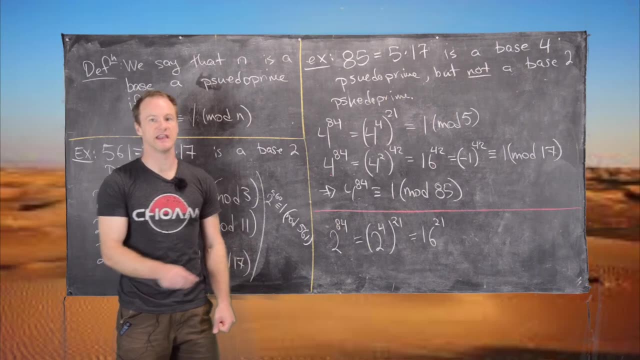 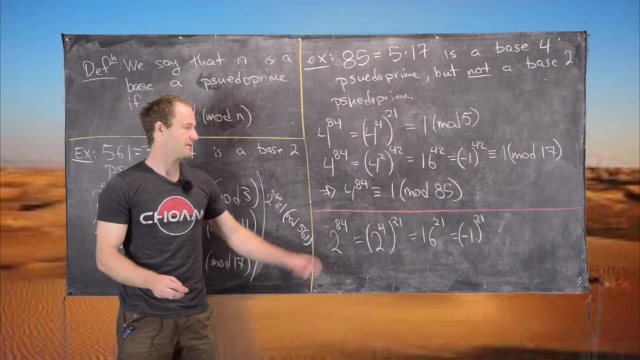 now 2 to the 4 is equal to 16 to the 21, and now you can see where the problem is creeping up again. you can see where the problem is creeping up again. you can see where the problem is creeping up again. 16 is congruent to negative 1 mod 17. so here we have negative 1 to the 21 mod 17. but now we have 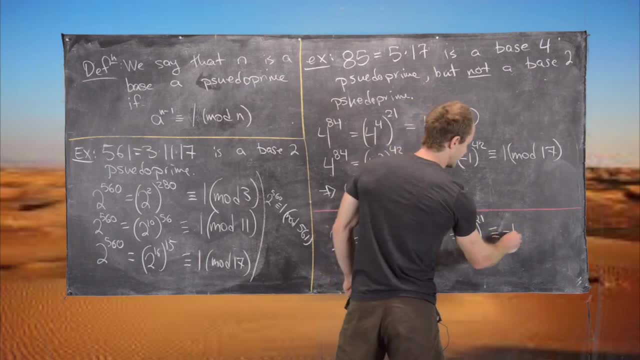 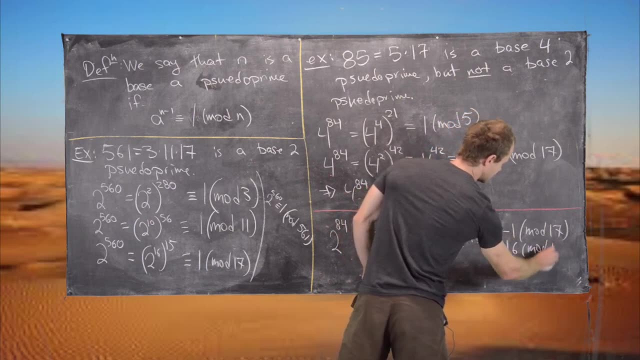 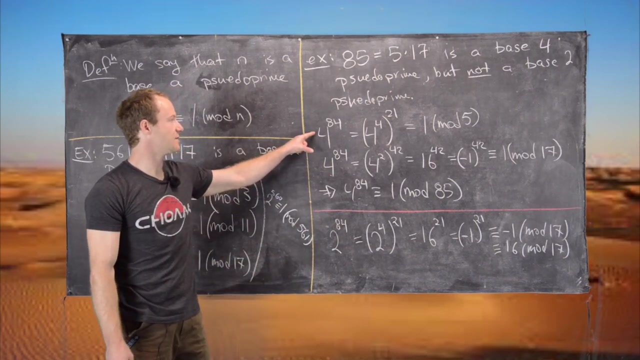 negative 1 to an odd power, which is clearly going to be negative 1 mod 17, which is itself 16 mod 17. good, so now, in fact, we can put this together. I won't check, but you can check that 2 to the 84 is. 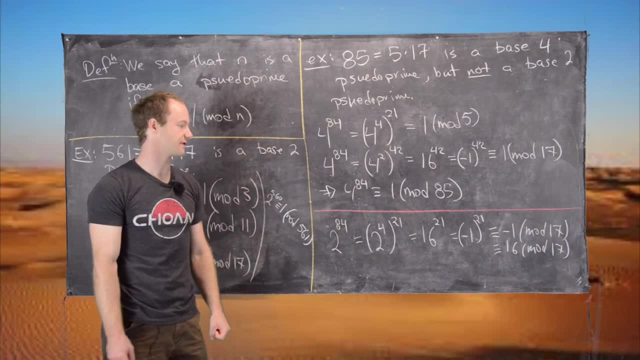 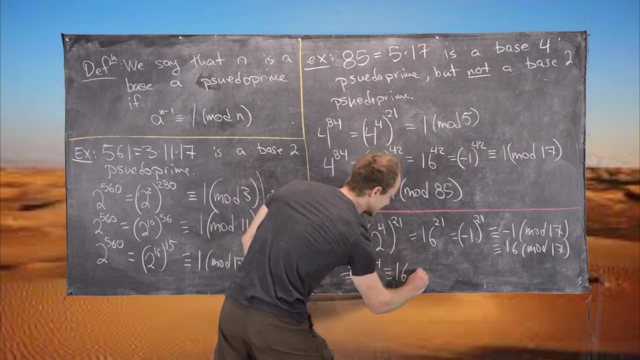 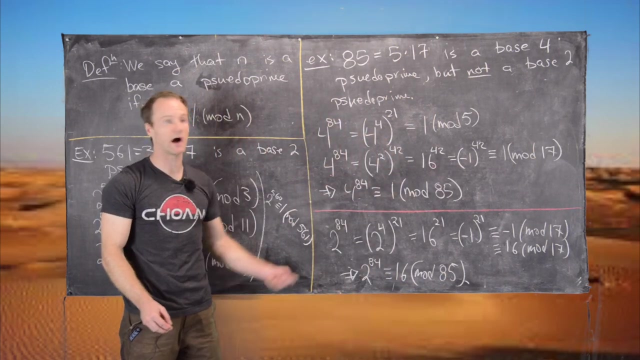 congruent to 1 mod 5. you can use the same trick with Fermat's little theorem, and so in fact what we have is 2 to the 84 is congruent to 16 mod 85, which is not 1 mod 85, so that means it's not a base. 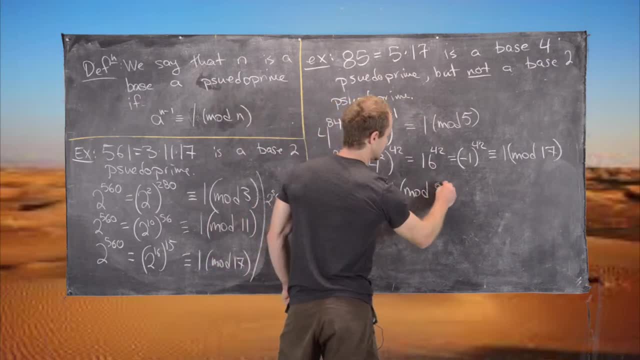 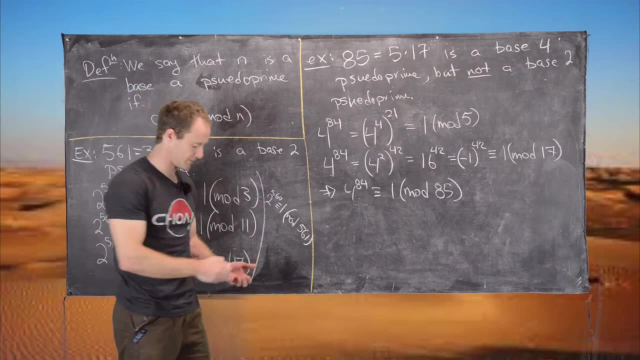 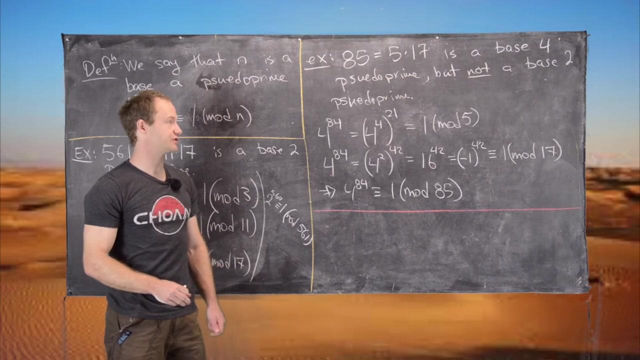 the product of 5 and 17,, which is 18,- sorry, 85,, which means that 85 is a base 4 pseudoprime. Okay, good, So now let's show why it's not a base 2 pseudoprime. So nothing will go wrong here. 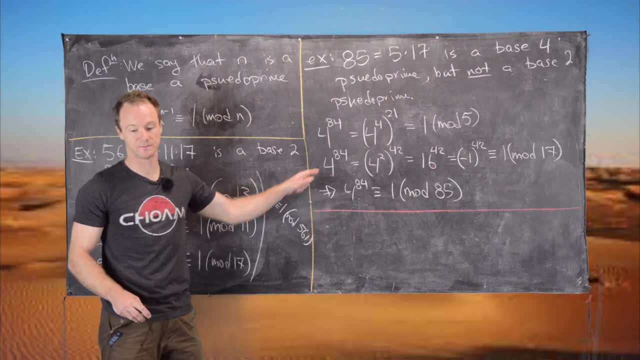 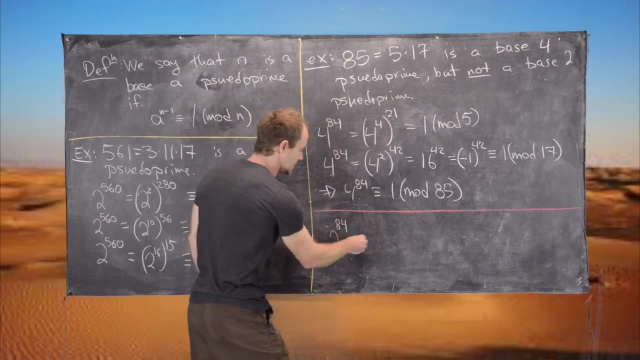 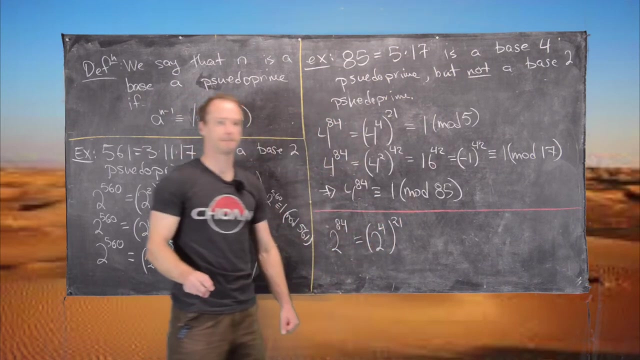 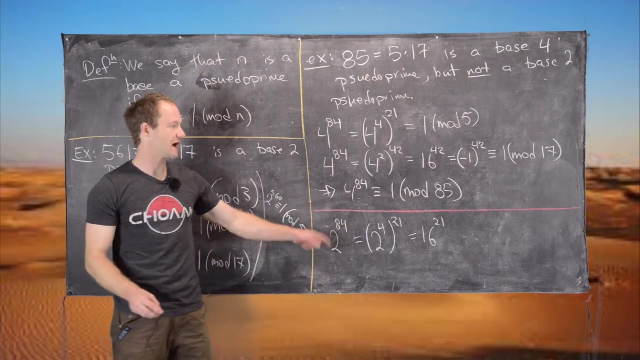 What will go wrong in this is in this, This type of equation. So now let's look at 2 to the 84, and notice that 2 to the 84 is equal to 2 to the 4 to the 21,. but now 2 to the 4 is equal to 16 to the 21,. and now you can see. 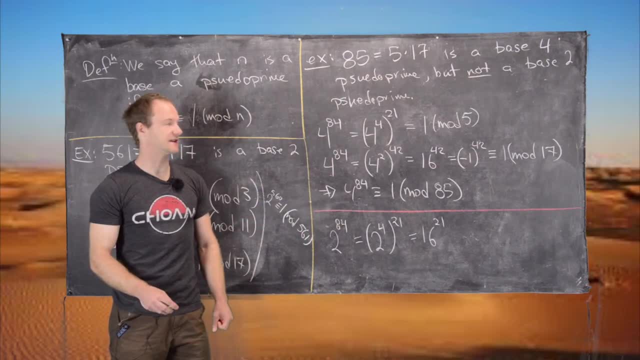 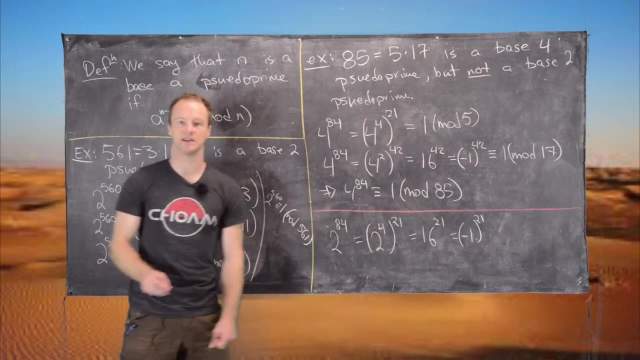 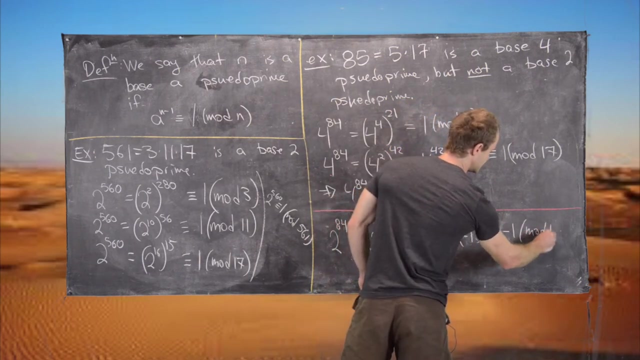 where the problem is creeping up Again: 16 is congruent to negative 1 mod 17,. so here we have negative 1 to the 21 mod 17,. but now we have negative 1 to an odd power, which is clearly going to be negative 1 mod 17,, which is itself 16 mod 17.. 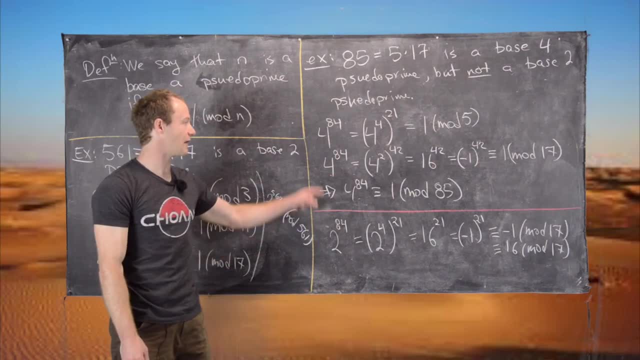 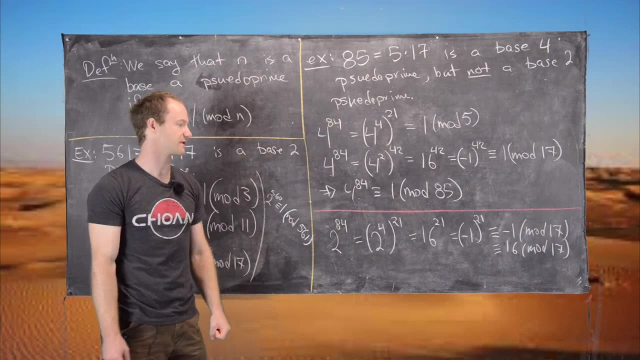 Good, So now in fact we can put this together. I won't check, but you can check that 2 to the 84 is congruent to 1 mod 5.. You can use the same trick with Fermat's Little Theorem. 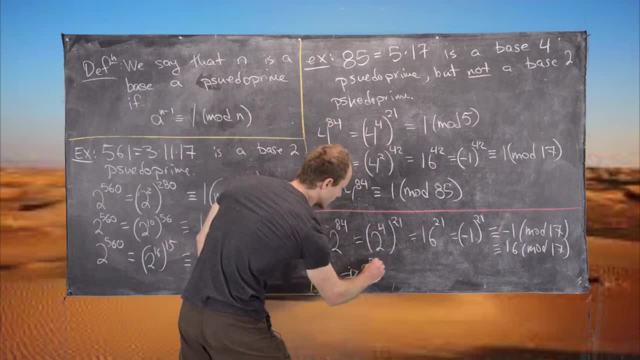 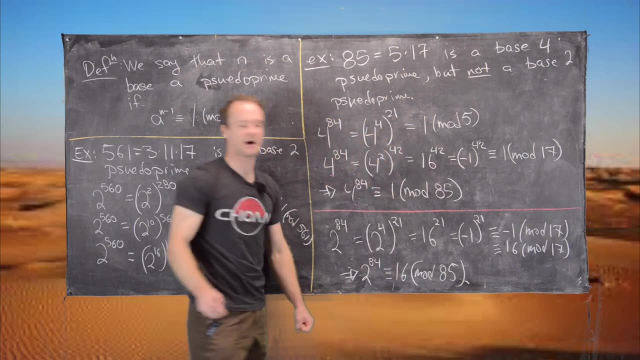 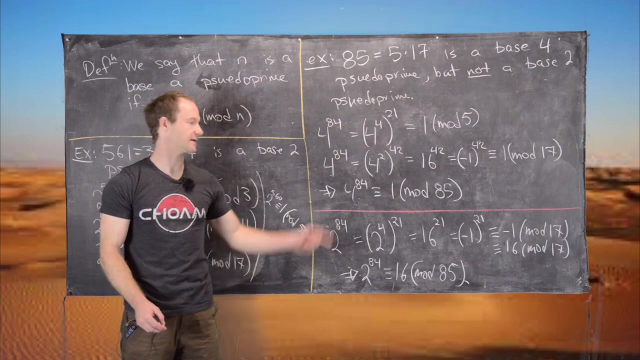 and so, in fact, what we have is 2 to the 84 is congruent to 16 mod 85, which is not 1 mod 85, so that means it's not a base 2 pseudoprime. Okay, this is the end of these examples. 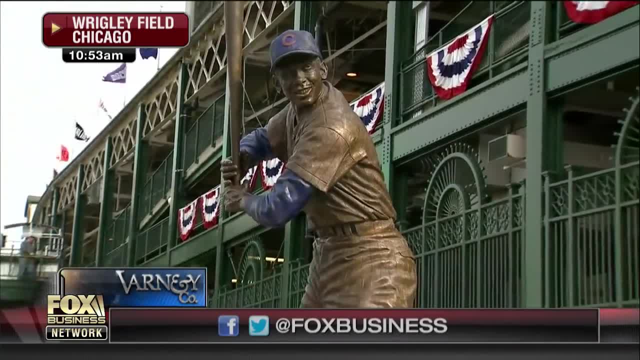 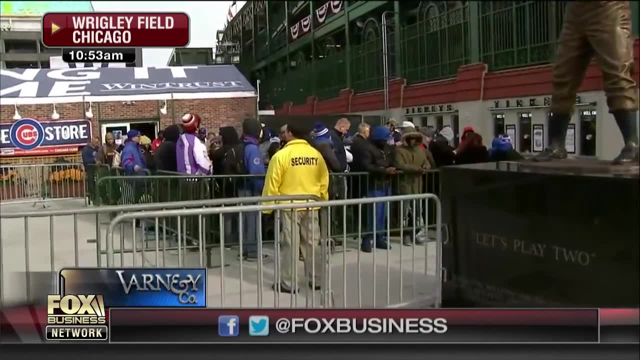 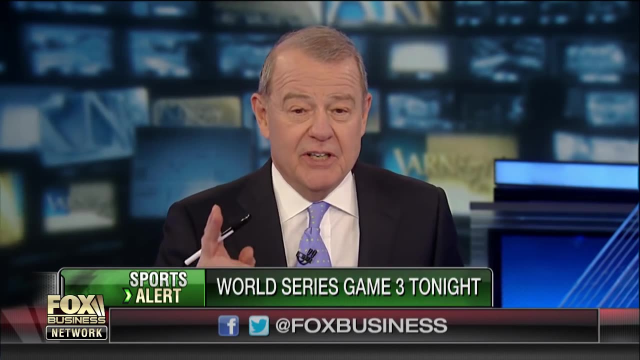 If I pitch, can you catch? Will you hold the ball Ratings for the World Series game tonight in Chicago? It's on Fox, of course. so yeah, it will definitely be record ratings. I will guarantee that there will be more people watch. 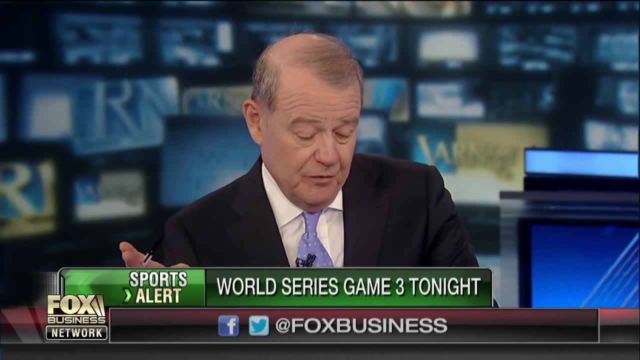 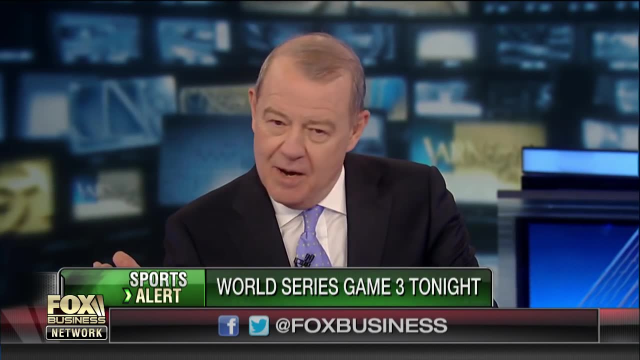 Game 3 of the World Series tonight from Chicago than watch that miserable football game between the Jaguars and the Titans last night on Thursday Night Football. Am I right or am I right? I think you are right. I'm perfectly right. Jeff Flock is there. The script says he's.